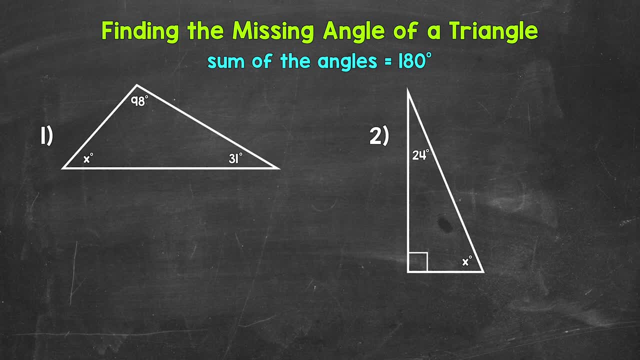 We need to know this information in order to find a missing angle measure of a triangle. Let's jump into our examples, starting with number one, where we have a triangle with a 98 degree angle, a 31 degree angle, and then x represents the missing angle measure. 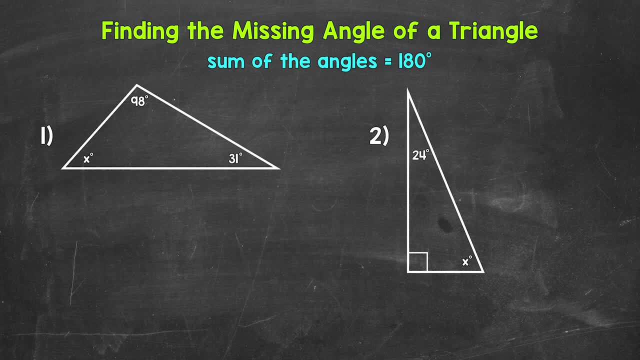 So how do we go about this? Well, we know that these three angles need to add up to 180 degrees. So let's set up an equation In order to solve for x. So we have 98 degrees plus 31 degrees plus x equals 180 degrees. 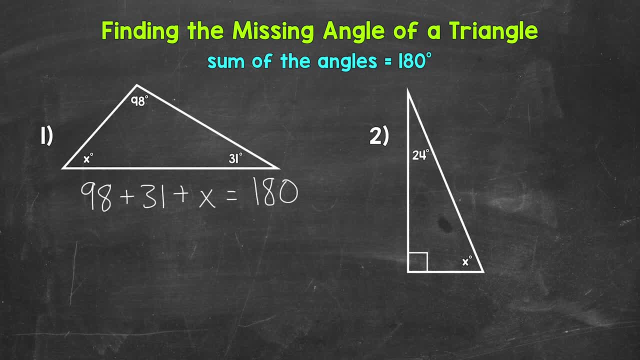 Now let's figure out what x equals. So we need to solve for x. Let's start by adding the two angles that we are given, So 98 degrees plus 31 degrees, That gives us 129 degrees. plus x equals 180 degrees. 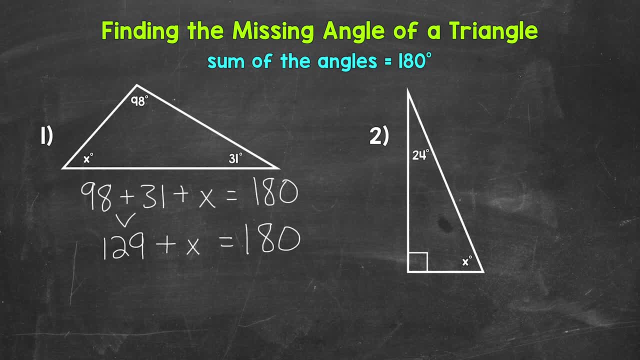 Now we need to isolate x. We need to figure out what x equals. We do this by subtracting 129 from the left side of the equation. Whatever we do to one side of the equation, we must do to the other in order to keep it balanced. 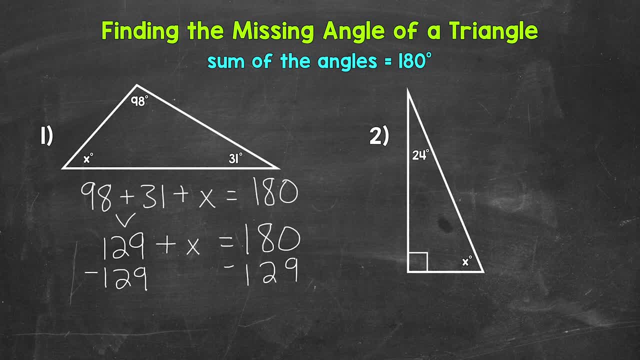 So let's subtract 129 from the right side as well. The 129s on the left side of the equation cancel each other out. So x is now isolated, x equals. And then, on the right side of the equation, 180 minus 129 gives us 51.. 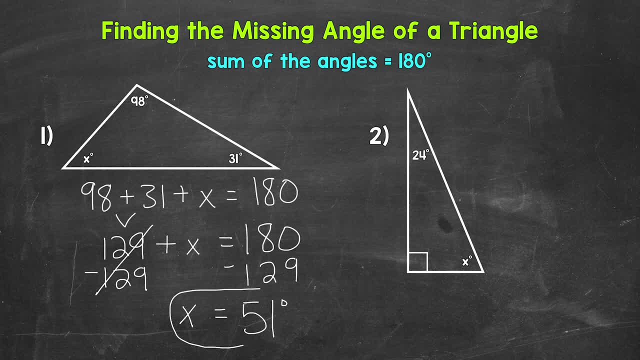 And this is degrees. So x equals 51 degrees. So that means that this missing angle measure is 51 degrees. Now we set everything up as an equation and worked through that equation in order to solve for x, But essentially all we did was add the two angle measures that we were given and then we subtracted that from 180 degrees in order to find the missing angle measure. 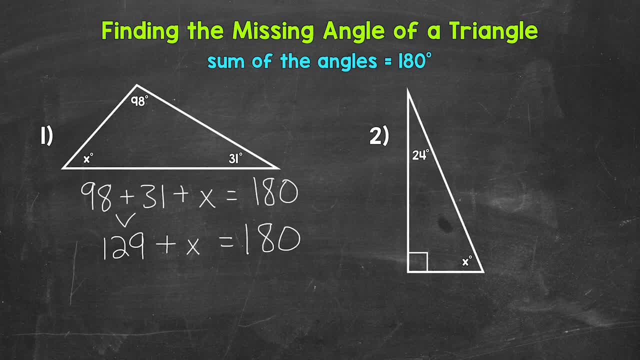 Now we need to isolate x. We need to figure out what x equals. We do this by subtracting 129 from the left side of the equation. Whatever we do to one side of the equation, we must do to the other in order to keep it balanced. So let's subtract 129 from the right side as well. The 129s on the left side of the equation cancel each other out. So x is now isolated. x equals... And then on the right side of the equation, 180 minus 129 gives us 51. 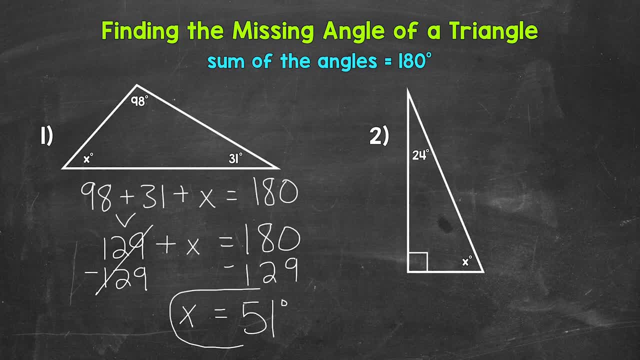 And this is degrees. So x equals 51 degrees. So that means that this missing angle measure is 51 degrees. 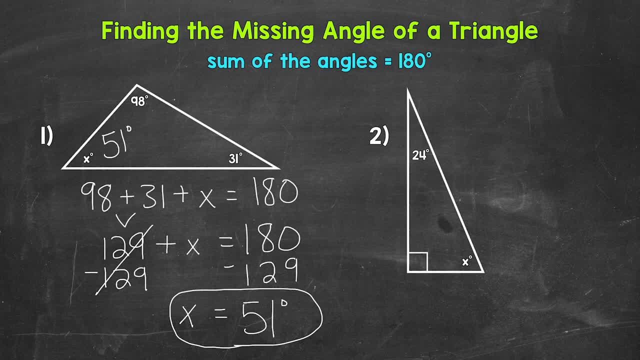 Now we set everything up as an equation and worked through that equation in order to solve for x. But essentially all we did was add the two angle measures that we were given and then we subtracted that from 180 degrees in order to find the missing angle measure. 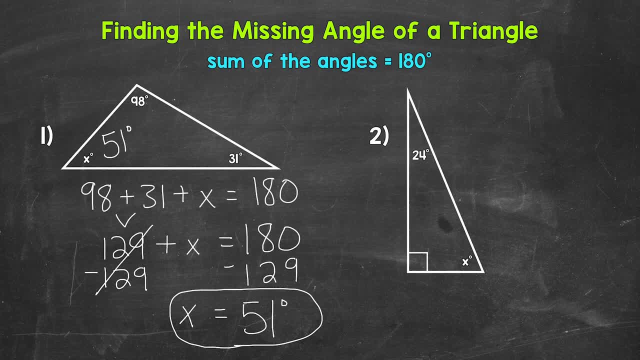 Let's move on to number 2 where we have a triangle with a 90 degree angle, a 24 degree angle, and then x represents the missing angle measure. Let's set this up as an equation and work through it in order to figure out what x equals. So we have 90 degrees plus 24 degrees plus x equals... equals... 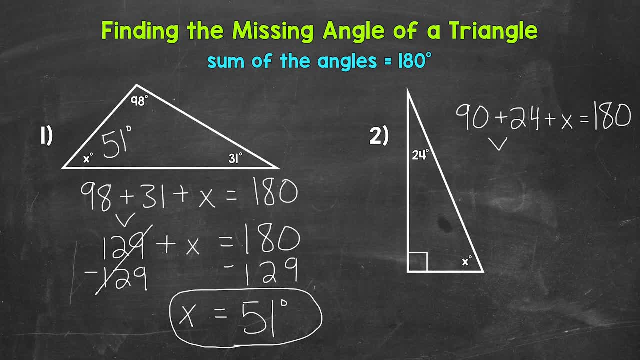 Let's start by adding the two angles that we were given. So 90 degrees plus 24 degrees. That gives us... 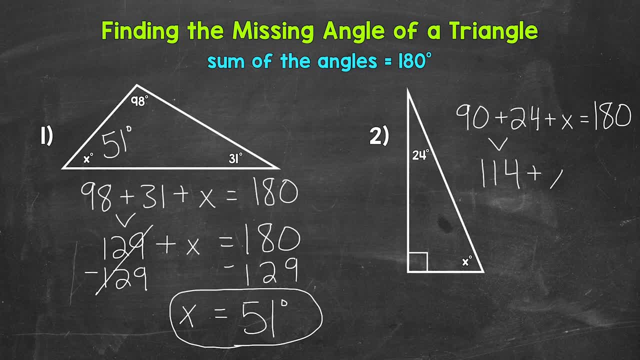 114 degrees... plus x... equals... 180 degrees. Now we need to isolate x. 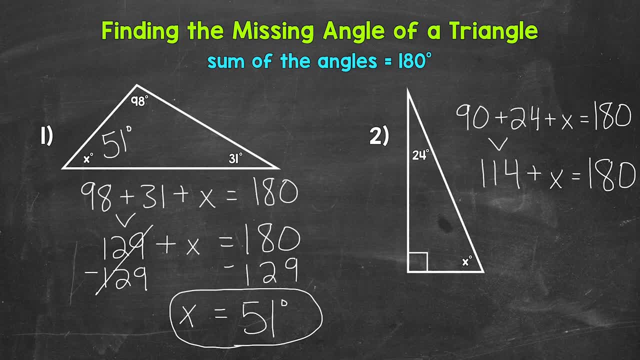 We need to figure out what x equals. So let's subtract... 114... from the left side of the equation. Whatever we do to one side of the equation... we must do to the other. So subtract 114 from the right side as well. The 114's on the left side of the equation... cancel each other out.